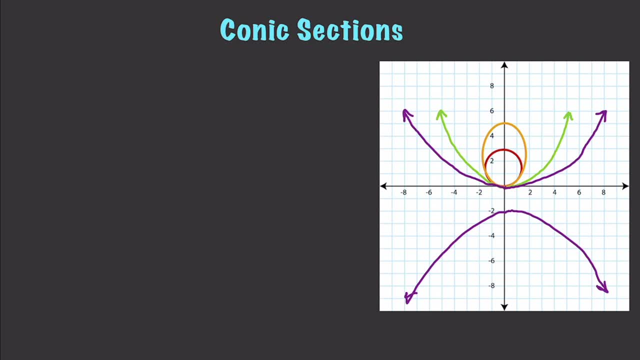 And throughout the next couple videos, I'm going to show you a whole bunch of tricks to create them, But I'm going to start off simple this time and talk about circles. Okay, so let's say that we have a conic section, So we have a point at 1- 5 and another point at negative- 2- 1, and what we want to do is find the distance between these points. 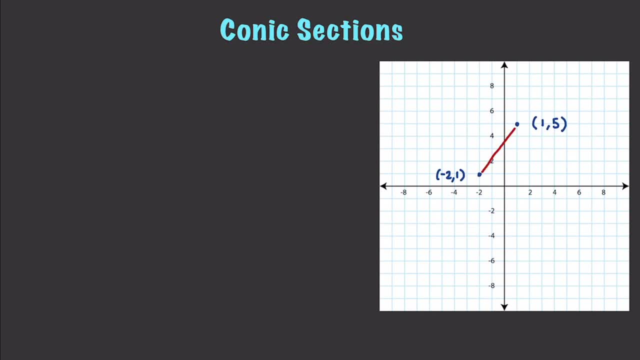 So what we would need to do to do this is to find out this distance right here, the height, which is going to end up being 5 minus 1, which is equal to 4.. And this distance right here, which is going to end up being: 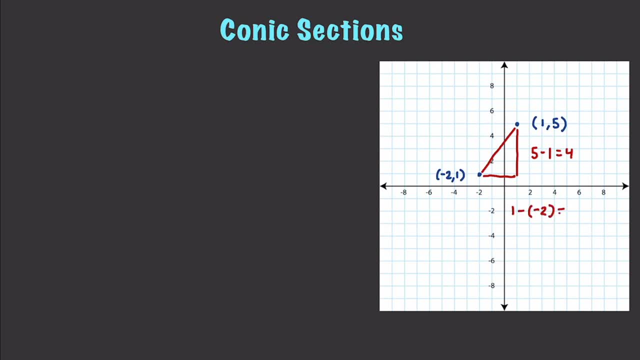 1 minus negative 2 or 3, and basically what we're going to use is the Pythagorean theorem as a guide, And the Pythagorean theorem, of course, is going to be: a squared plus b squared is equal to c squared, And in that situation, this is the c part, this is the a part and this is the b part. 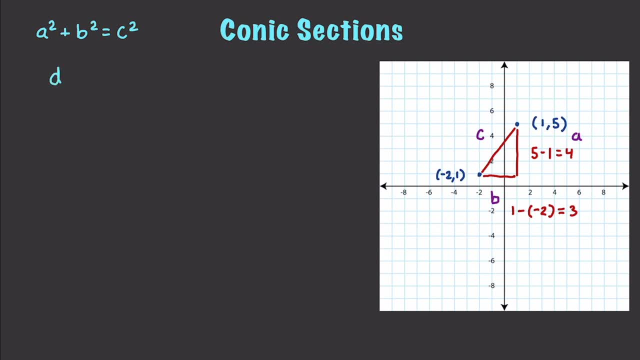 And we're specifically going to use this formula: distance is equal to x2 minus x1 squared, plus y2 minus y1 squared, and then, of course, find that square root. so this, of course, is going to end up being exactly what I just showed you on the right, but I'm going to put it in the proper form, so it's going to be 5 minus 1. 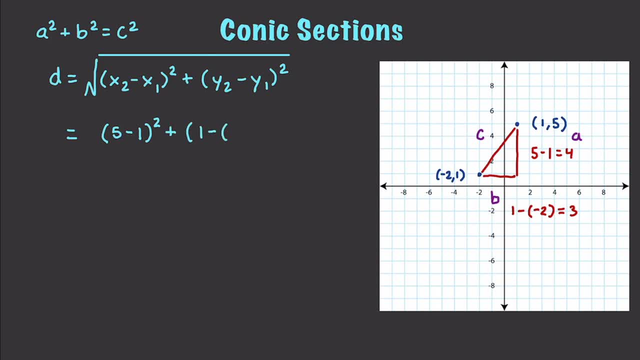 squared plus 1, minus negative, 2 squared, and then we'll find that square root which is going to end up being 16 plus 9, which, of course, is going to be equal to the square root of 25, or simply 5.. You're also going to be able to find the midpoint of these two points. so we're talking about a point. 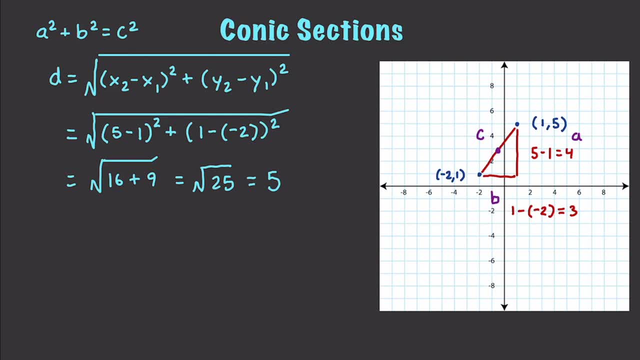 that is going to lie somewhere in the middle of the square root of 25. Somewhere in this area. and how we're going to find that is we're going to have x1 plus x2 divided by 2 and y2, and y1 plus y2 also divided by 2, which is going to end up being negative 2. 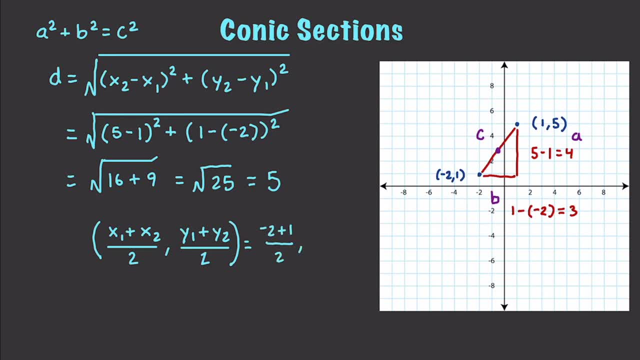 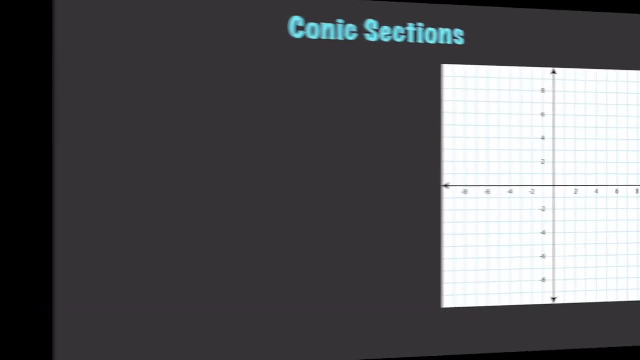 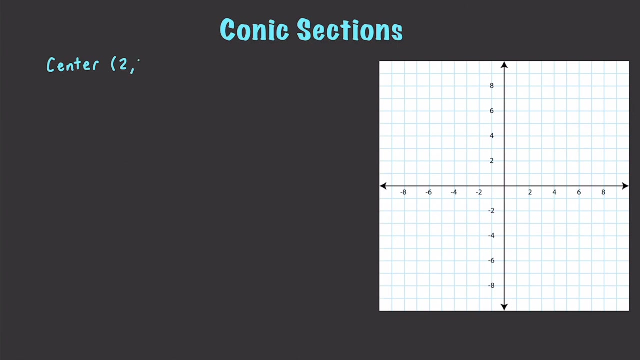 plus 1 over 2 and 1 plus 5 over 2, to get a final midpoint of negative 1, half and 3.. Alrighty, and now I'm going to work out a couple plots here. Now let's say that we have a circle and its center point is known to be at 2- 4, and say that we also 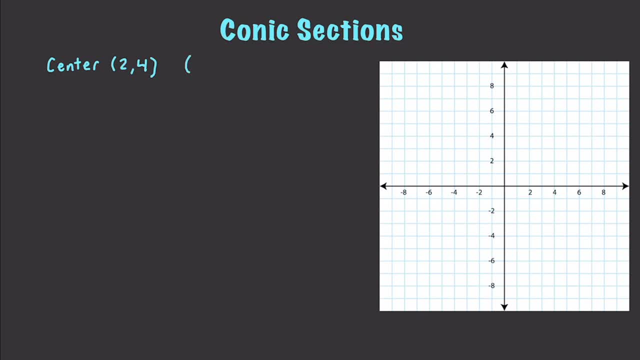 have two additional points being negative: 3 and 4, as well as 7 and 4.. Well, we're going to be able to calculate our diameter for our circle and also then get the radius. so this is going to be diameter in this situation, and this is going to work out to be 7 minus negative 3, and this is going to be. 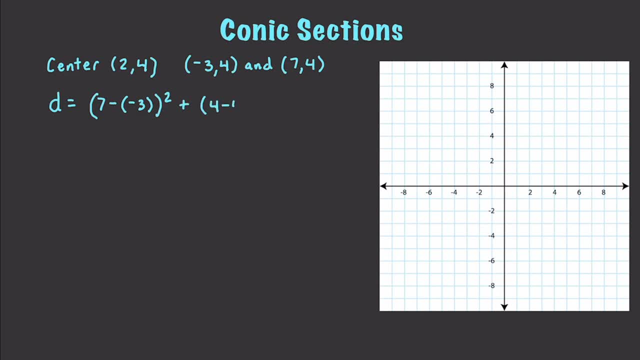 squared, plus 4, minus 4 squared, we will then take the square root of that which is going to end up being equal to 10 squared square root, which, of course, they cancel each other out, And you would get a final diameter of 10, and then, to calculate our radius, you would get a 10 over 2 or 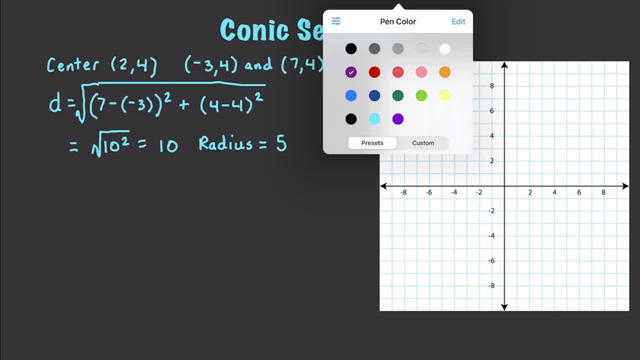 just simply 5 and of course we could easily plot this. we know our center point because it's right here, so that's going to be 2 and 4. so there is our center point and we know our radius, which is going to be equal to 5. so that's going to put a point out here, a point over here, a point up here. 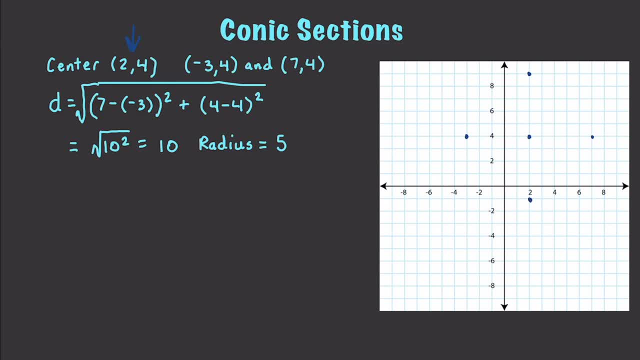 at 9.. A point down here at negative 1, and then we could just come in here and the best that I can, I will draw in our circle, and there you go is a rough estimate of what that circle would look like. now, of course, we do not need all of those points to be able to plot a circle, and this is the basic formula. 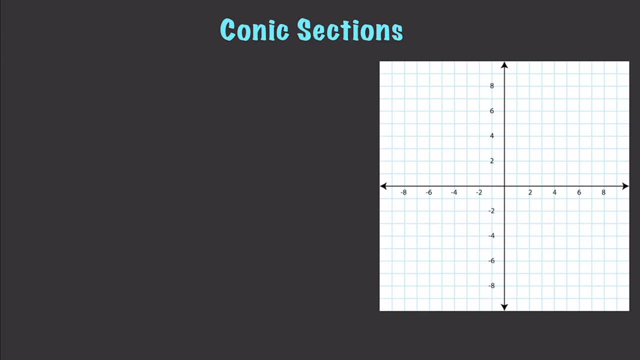 for a circle. if you have a center point of H and K with a radius R, then your formula is going to be X minus H squared plus Y minus K squared is equal to R squared. and let's say you have a central center point for your circle and you know that it is 1- 2 and you also know that you could mark this as: 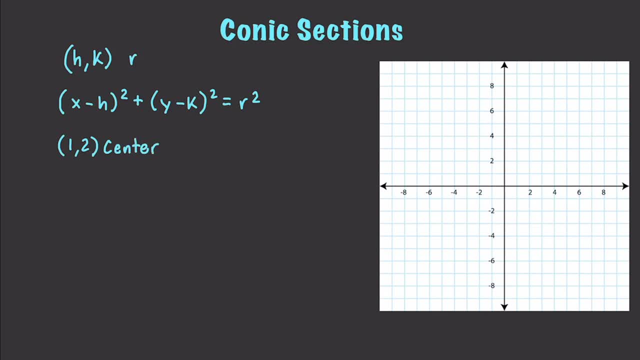 center, and you also know that there is an additional point at 5: 2. well, to calculate our radius, Once we have our radius, we're going to be able to plot a circle, and then we're going to have a circle again. it's going to be radius this time. this is going to work out to be 5 minus 1 squared. 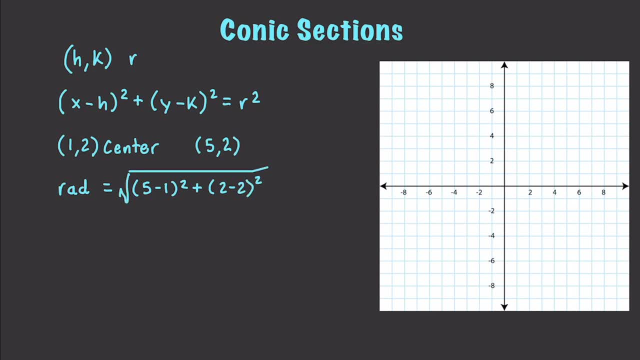 plus 2, minus 2 squared. take the square root of that, which, of course, is going to end up being equal to 4 squared square root which just cancels out to be 4. so now we know our radius is 4.. We can then take our formula, which is this guy right here. 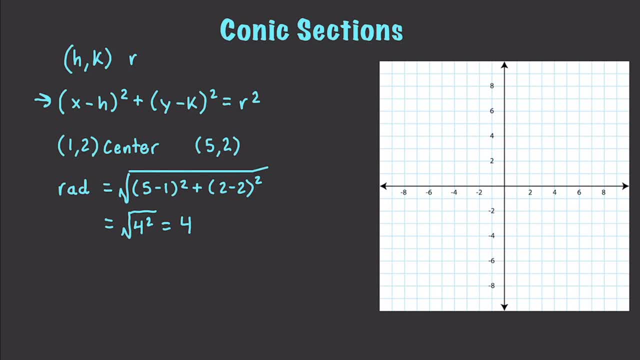 and we can plug in our center points as well as our radius. so I'm just going to write this up here: the radius is equal to 4, so this is going to do change- and our center point- we'll just write this as center- is equal to 1: 2. this then becomes X minus 1 squared plus Y minus 2 squared, which is 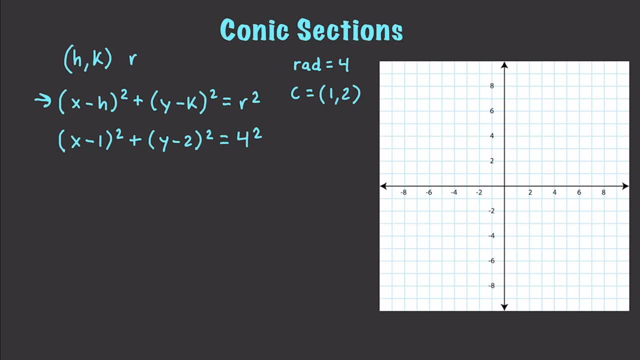 equal to 4 squared, And then we could do interesting things like, let's say, we tried to find the X intercept, so the points in which our circle would hit the X axis, or something like that. why don't we just go and plot this and then I'll show you how to do that, so we know what we're at. 1, 2. so 1, 2 right here and we. 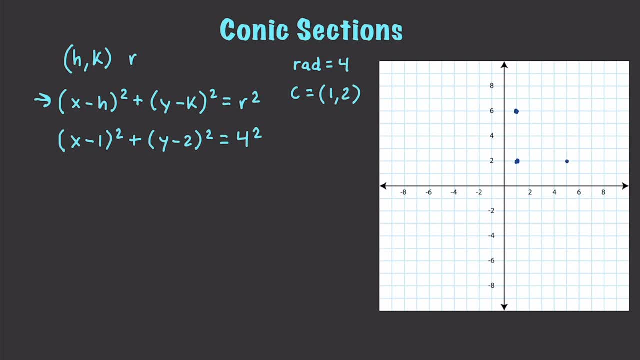 know, our radius is 4, so we have a point up here, a point over here, here here, and then come in and draw in our circle, and that's a little rough, but it should be clear, Close, and then let's say that we would want to find our X intercept. well, to do so, all we need to do 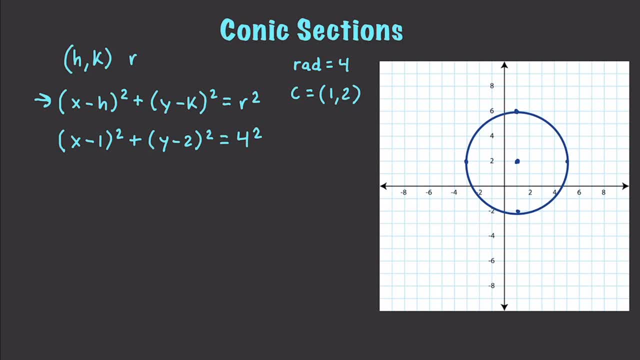 is plug in 0 where we have Y. with this formula we have right here. so this is going to end up being X minus 1 squared plus 0 minus 2 squared. you can see I put the 0 right there, like I said I was going. 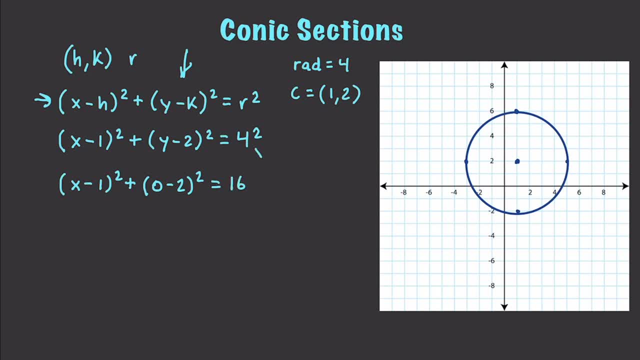 to, for Y is equal to 16. of course that comes from right there and this is going to say: we're going to simplify down to be: X minus 1 squared plus 4 is equal to 16, and then this is going to be translated into: X minus 1 squared is equal to 12 whenever we subtract 4 from both sides, and that is going to 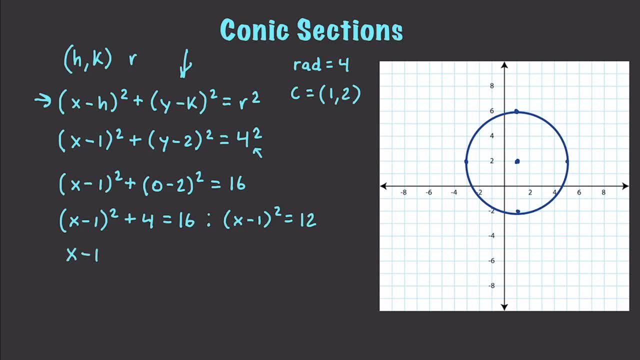 end up being equal to: X minus 1 is equal to the square root of 12, which is going the square root of 4 times 3, which is going to end up being equal to. if we take the square root of just 4, then we'll. 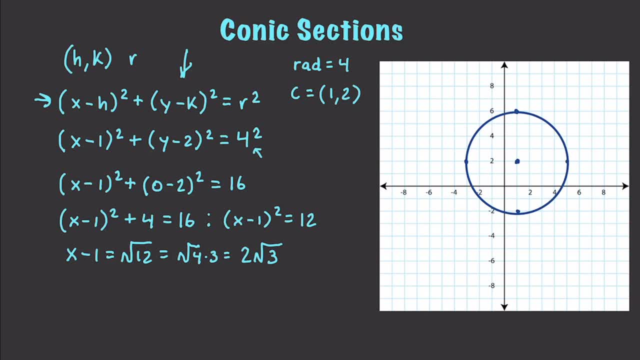 get 2, leaving 3 behind, and that means that, finally, X is going to have a value of plus or minus 2 square root of 3 plus 1, and then that works out to being an X1 equal to X minus 2 squared plus 1. 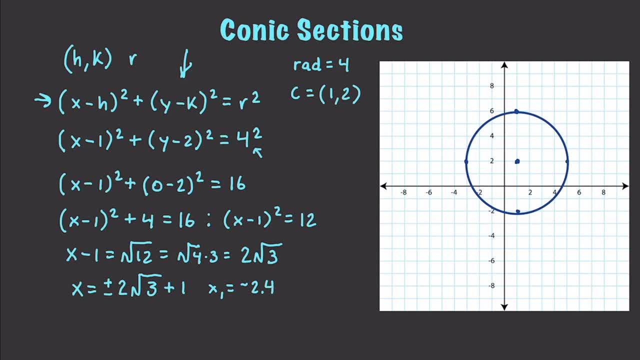 negative 2- this is an approximate value- 2.46 and X2 is going to have a approximate value of 4.46. and if we come in here and actually look, does this look like about 4.46 right here? that's doggone close. and does this look approximately like negative two and a half? yep, very close. and 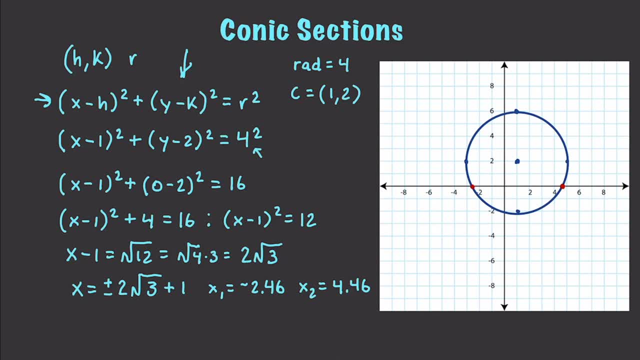 that's the circles off a little bit, all right. so there is an introduction to quantic sections and more specifically, just graphing circles, because we haven't covered that and I wanted to cover a whole bunch of other formulas in relation to working with circles and in the 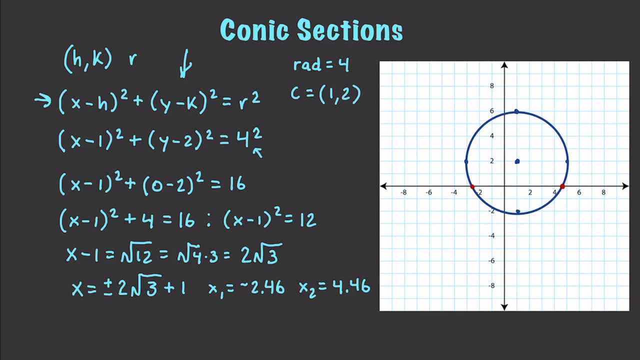 next video I'm going to cover parabolas and, like always, please leave your questions and comments down below. otherwise till next time.